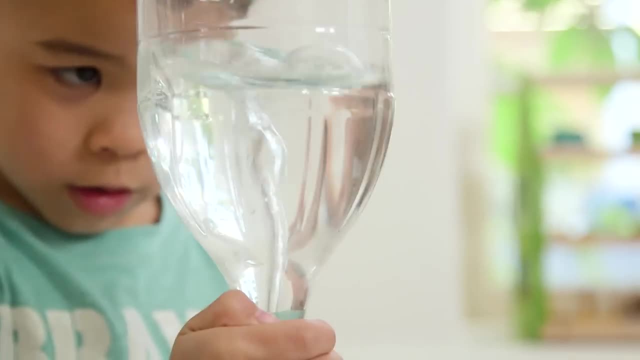 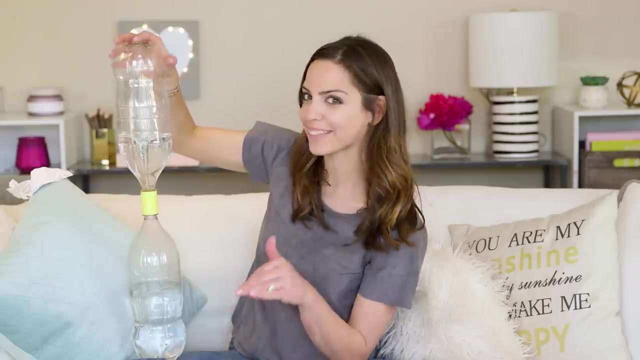 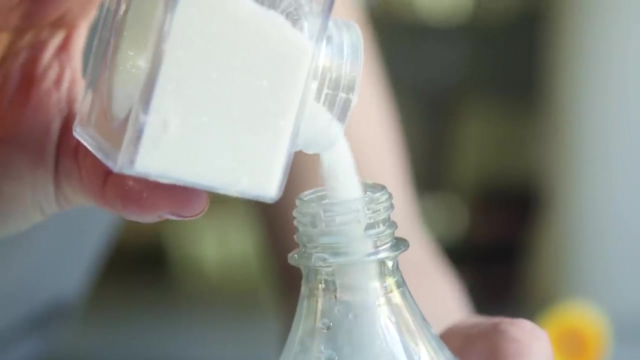 technically a vortex, but my kids loved it. It's kind of like watching your bathtub run out. They always wait for that moment. They won't get out before that. And you can add liquid, dishwasher soap and glitter for even more of a tornado effect. Oh, that's so pretty. Oh my gosh. 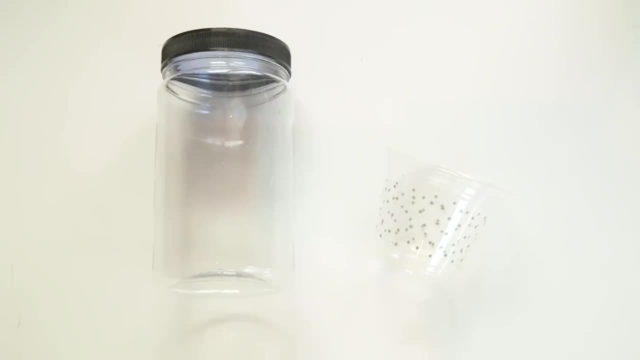 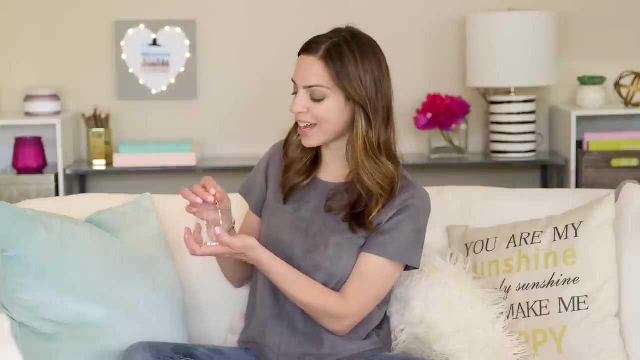 Next up raining cotton balls. You'll need a jar, a smaller clear cup, cotton balls and optional blue dye to give your water a little color. So you're going to want to start by poking holes in the plastic cup, Add some cotton balls and then place it into your bigger cup and pour. 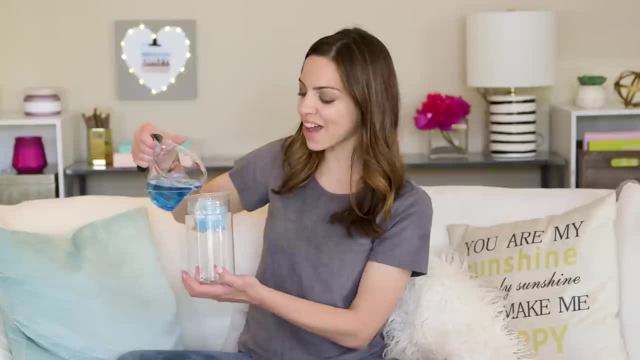 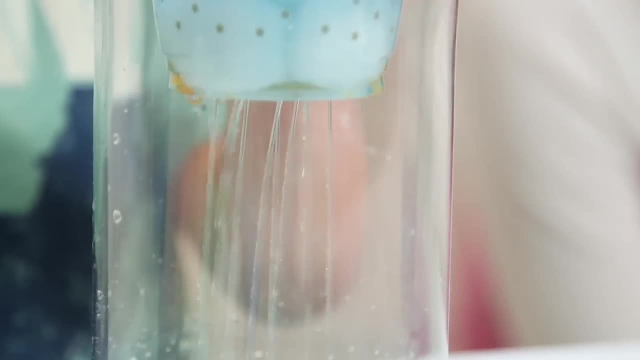 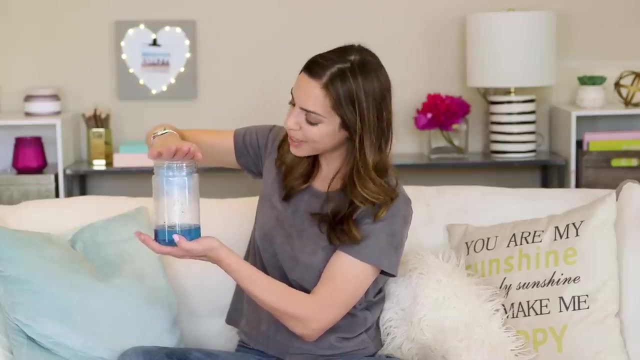 the water in, And as soon as the clouds are heavy enough, it's going to start to rain. And then it's a fun little twist: Put your hand on top of it and the rain stops, because the upward air pressure is actually stronger than when it was with the rain. So you're not going to get any water. 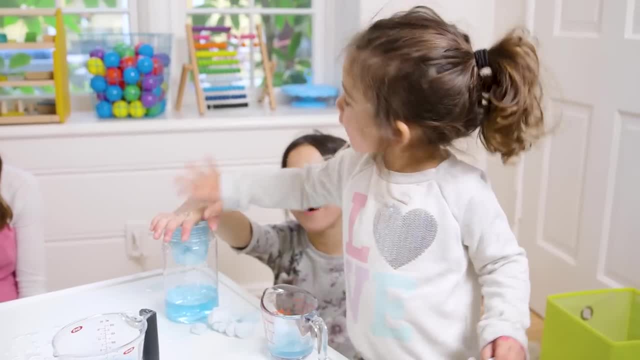 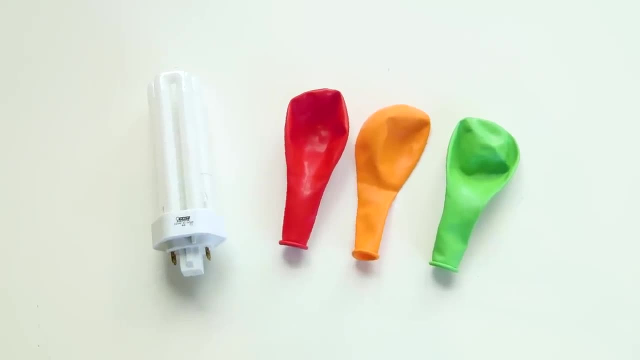 in there It's going to be a little bit more heavy, So I'm going to start with some cotton balls and actually, stronger than the gravity pulling the liquid down, release it and it goes again. Next up, static electricity lightning. You'll just need a balloon and a fluorescent light bulb. 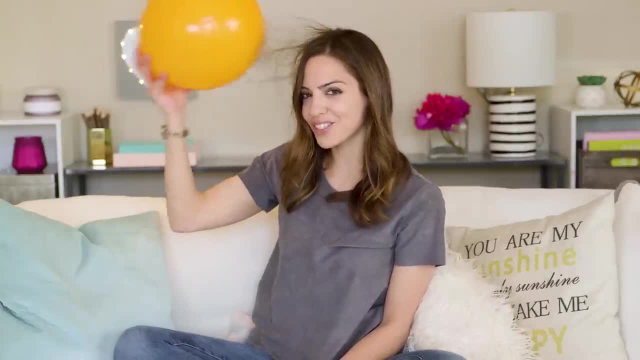 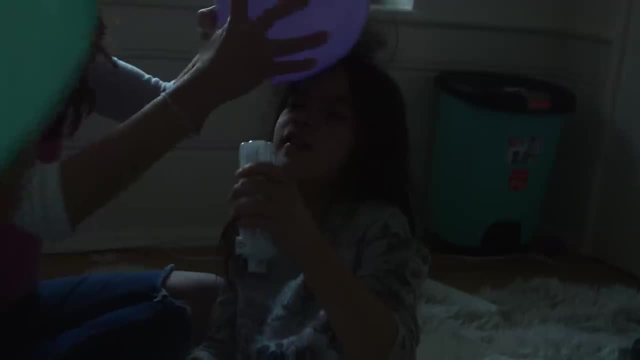 Start by rubbing the balloon on your head for two minutes, which builds up a negative charge. Rub the balloon in your hair, Turn off the light. put the two together and it's quick, but you'll see a flicker of light. 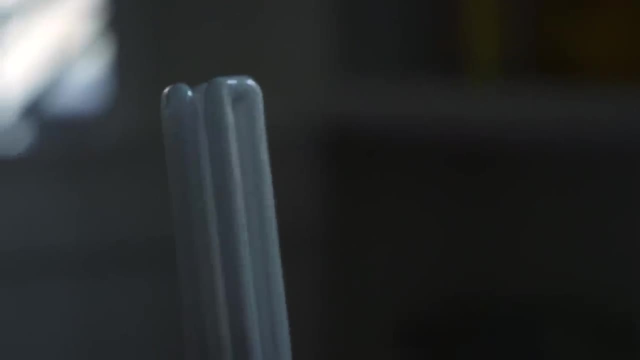 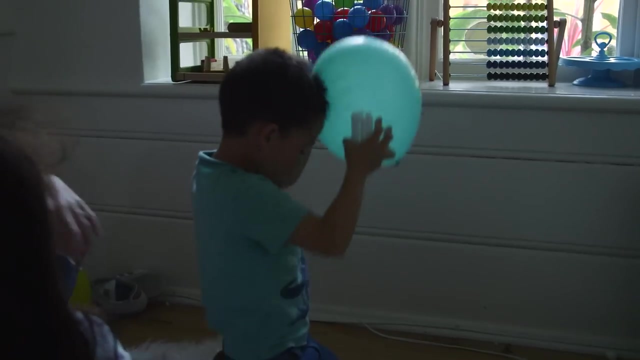 And what's happening is the positive ions are heading towards the balloon, the negative ones away, and they collide together, forming the light, similar to how lightning is formed. It's a little more complicated than that, but that's the best I can do. 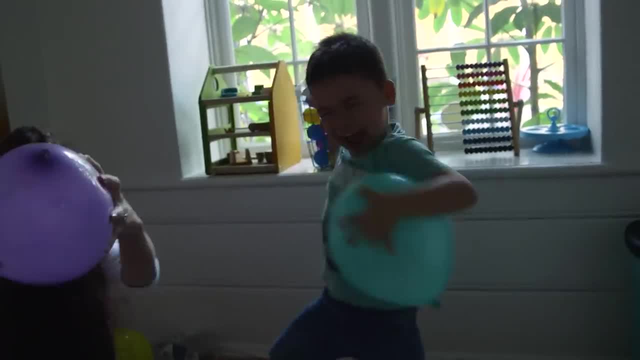 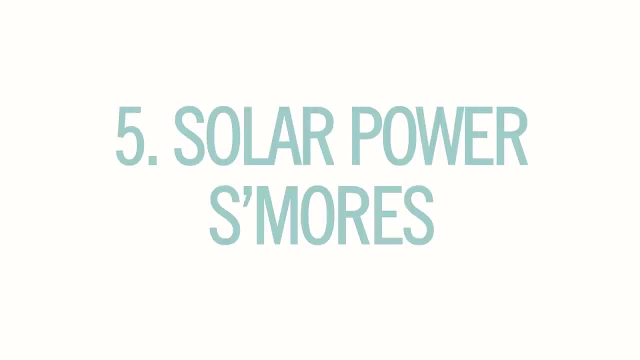 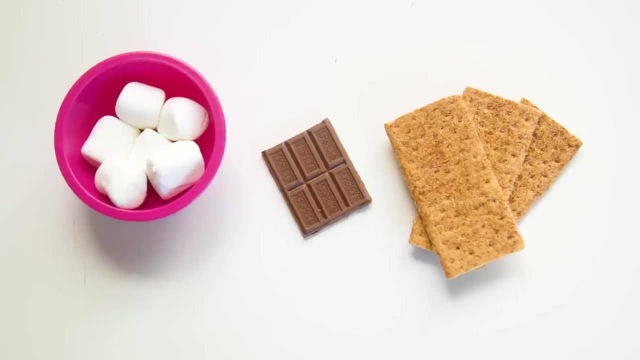 I did it. Oh yeah, Yeah, Yeah, yeah, yeah, I got a little more volume now. Next up we've got solar power s'mores. You'll need a pizza box, plastic wrap, aluminum foil, black paper and, of course, s'mores. 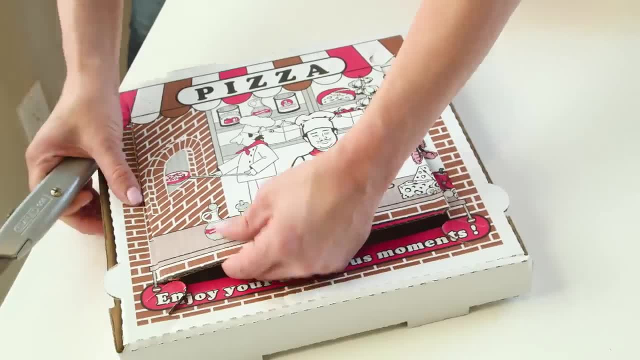 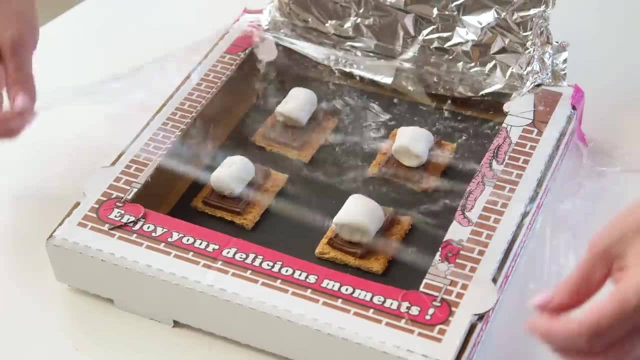 ingredients. Start by cutting a hole in the top of the box, lift that up and cover with aluminum foil, place the black paper inside the box, your ingredients on top, and cover that with wrap. So Tess and I did this earlier in the day and it worked awesome.